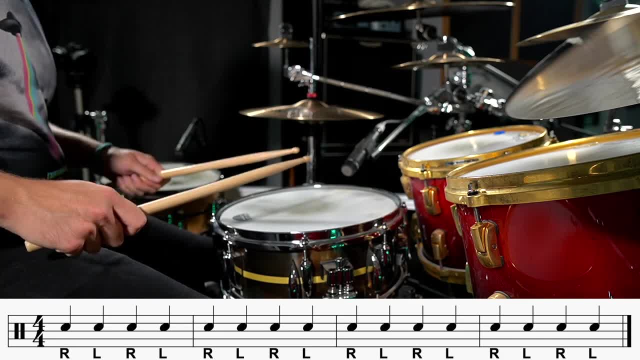 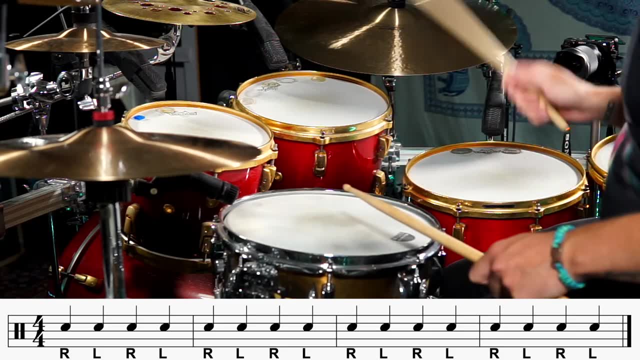 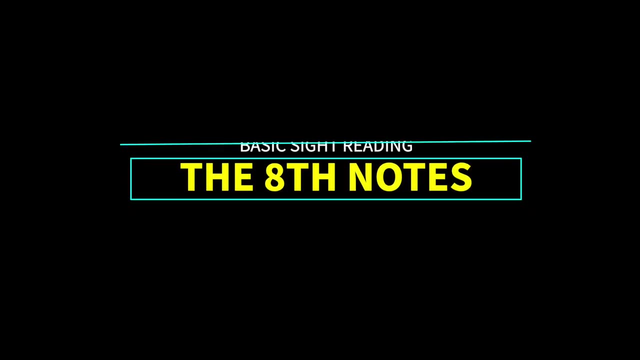 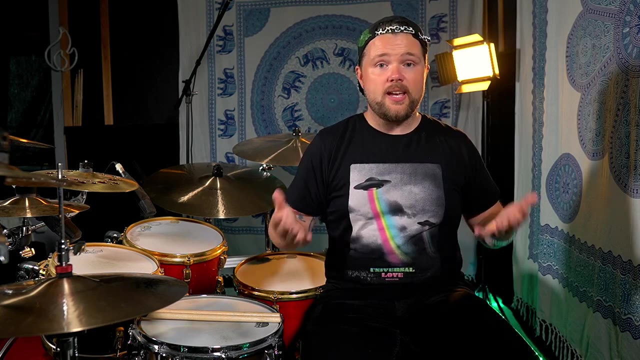 that wasn't so bad right. okay, let's move on to the eighth notes. eighth notes are quarter notes that has been split in two. so if you split four quarter notes in two, you get- you guessed it- eight, eighth notes, or if you're british you might call them quavers. 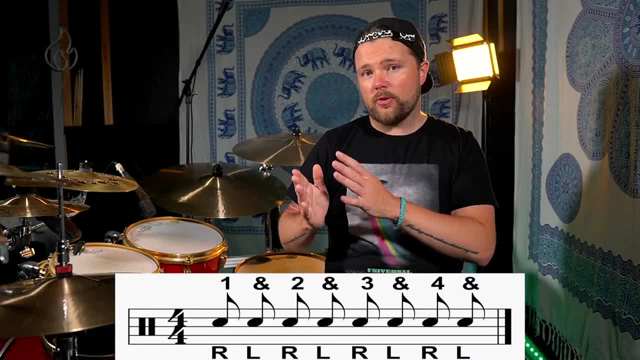 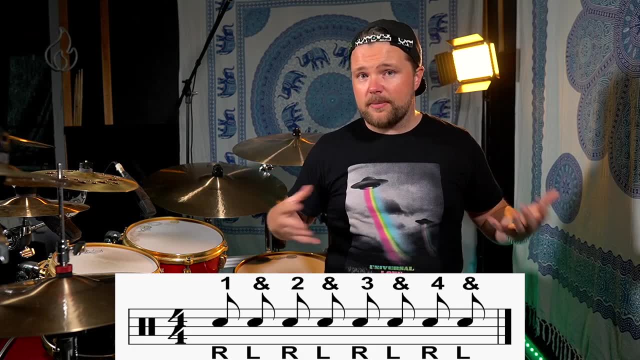 the transcription will show that the eighth notes look similar to the quarter notes, but now there's a small flag on top of the staff and instead of writing out eight individual notes with a flag on every measure, you can tie these together in groupings of two or four. with what in music? 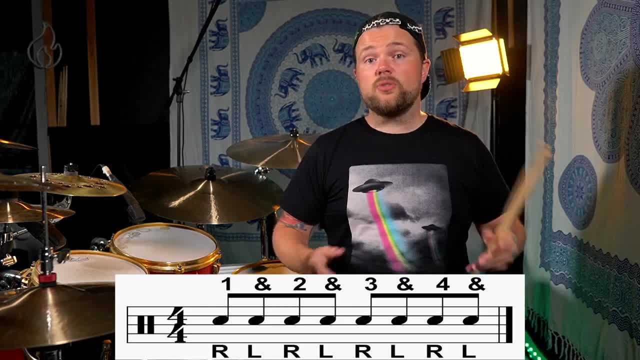 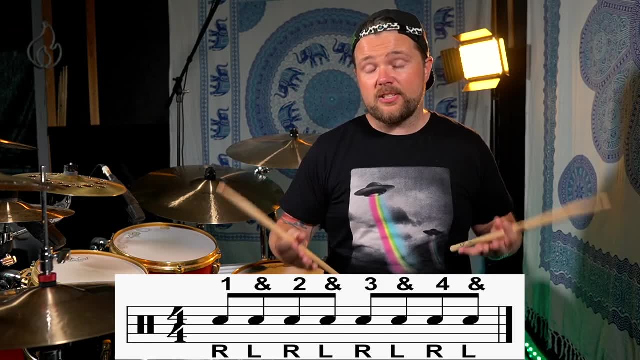 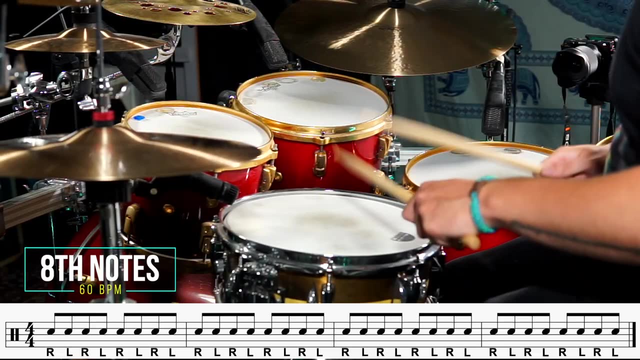 theory is called a beam. it's easier to read that way. eighth notes are counted as one and two, and three and four, and and of course the sticking is alternating right and left. let's try it out at 60 bpm and then at 90 bpm. so 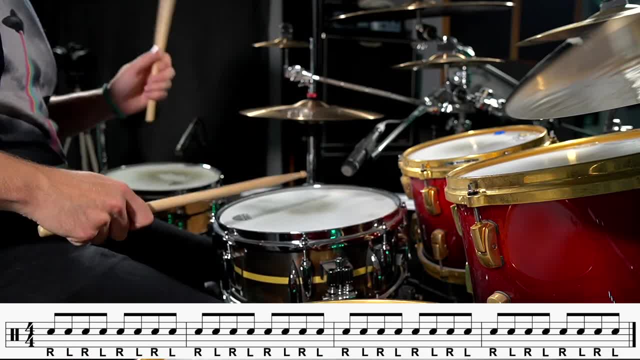 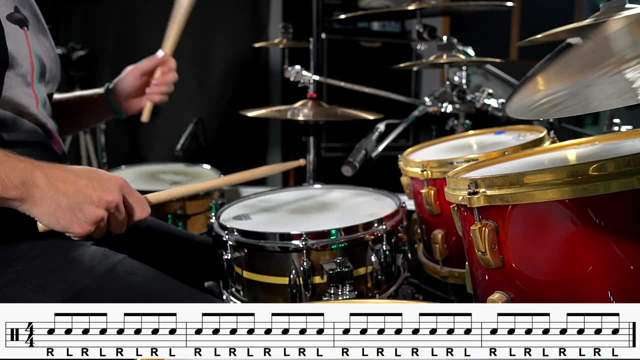 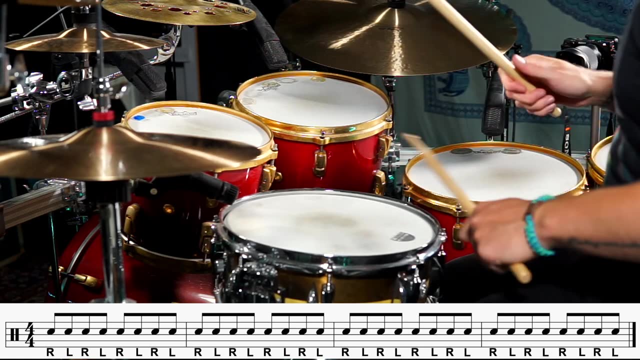 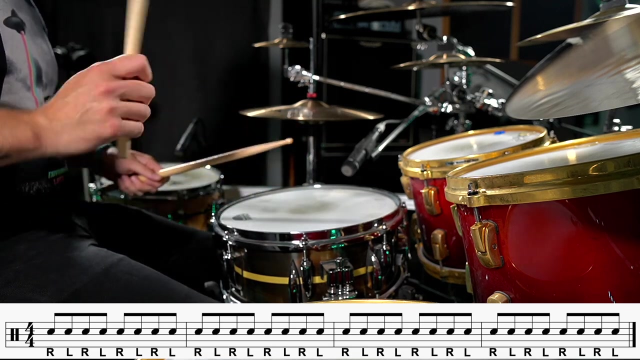 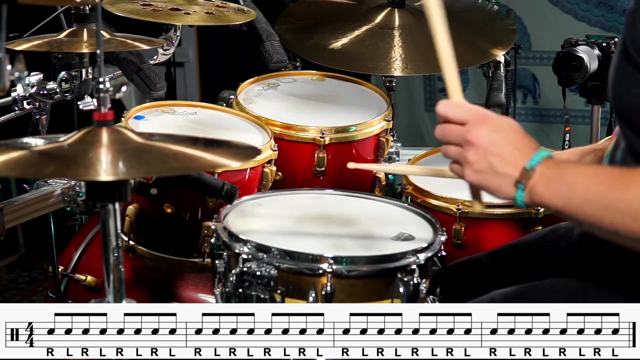 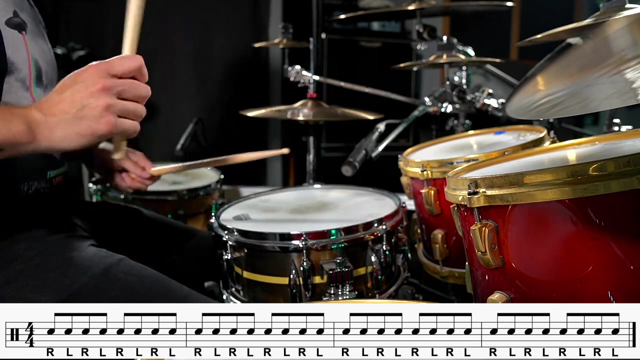 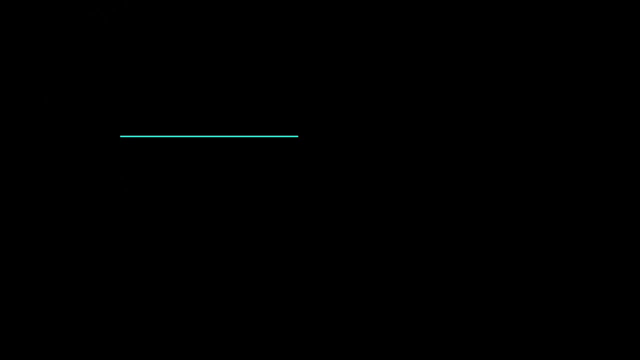 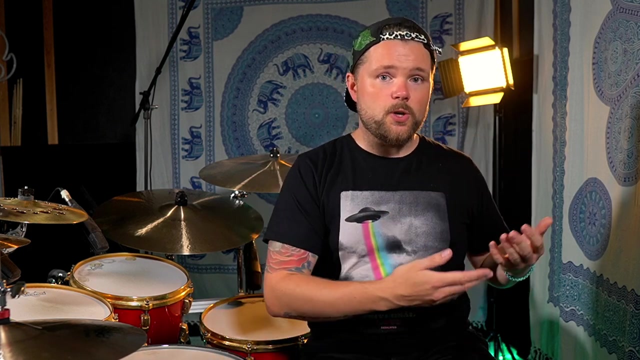 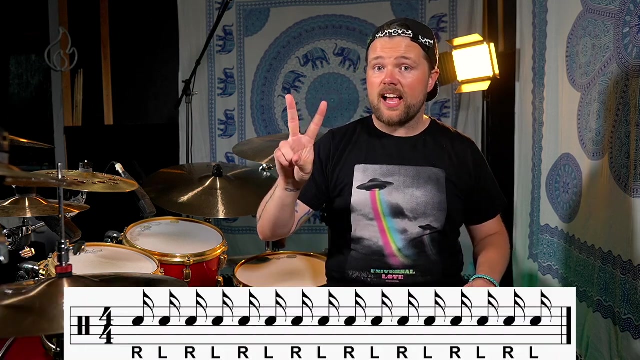 16th note. 16th note: Korean 16 d. both notes sum BC new ny. sixteenth notes. As you can see, the sixteenth note has two flags on the staff And since one quarter note is worth four sixteenth notes, we write them. 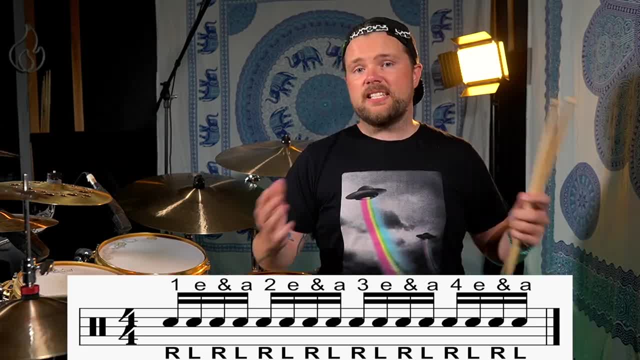 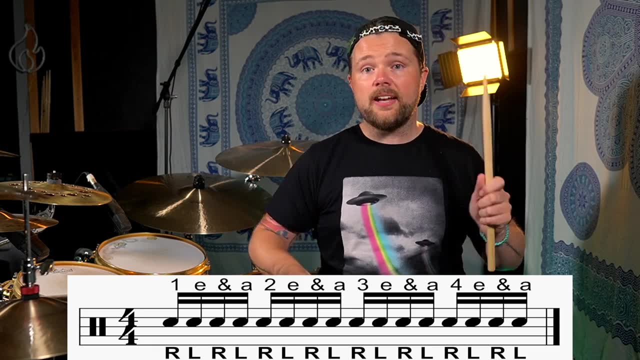 out in groupings of four with two beams that tie them together. Sixteenth notes are counted as one E and a two E and a three E and a four E and a one, And of course the sticking is right left, right left. Let's try them out. 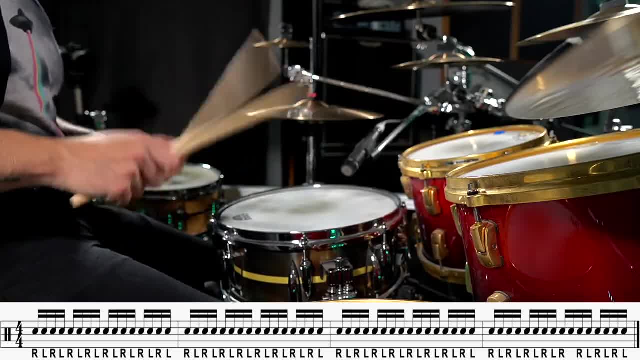 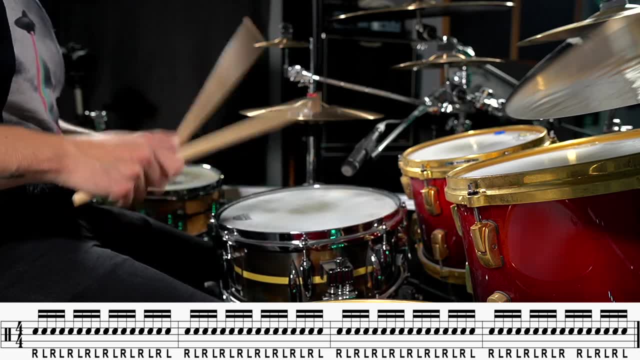 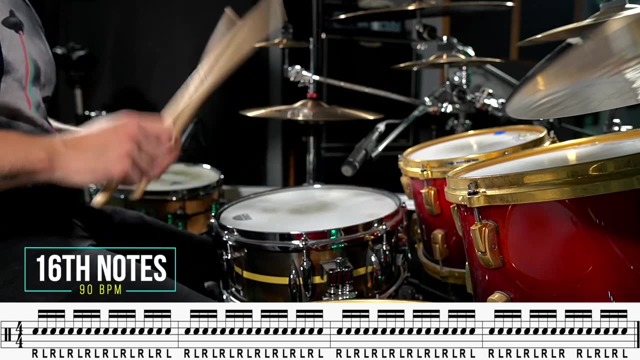 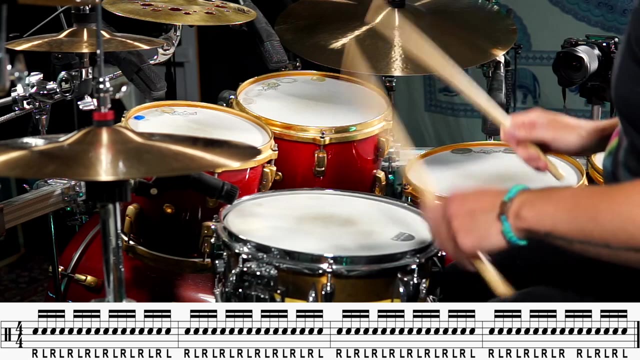 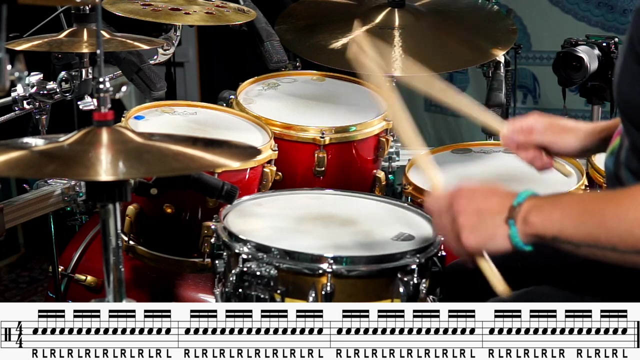 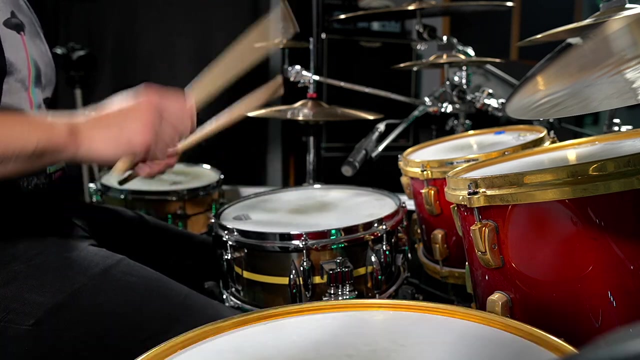 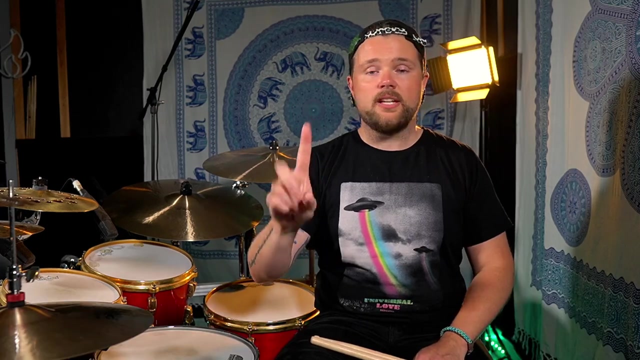 Awesome work, you guys. Now I'm going to show you some combinations of these different note values and how to count them. The first is one eighth note and two sixteenth notes tied together. As you can see, the eighth note is linked together. 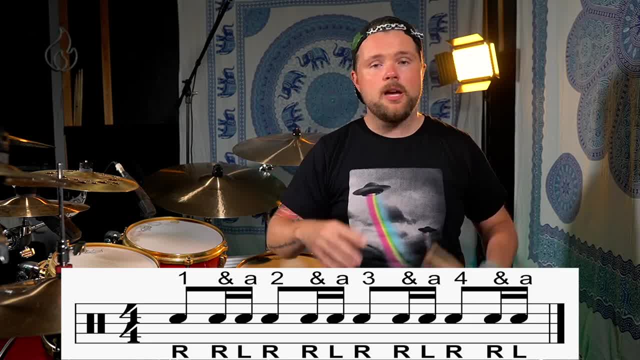 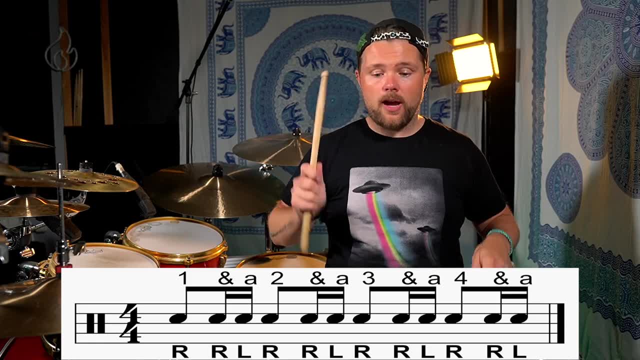 with one beam to the two sixteenth notes. that has two beams marking them as sixteenth notes. When you count this out, you go one and a two and a three and a four and a one. And to make it even easier for the complete beginners or when 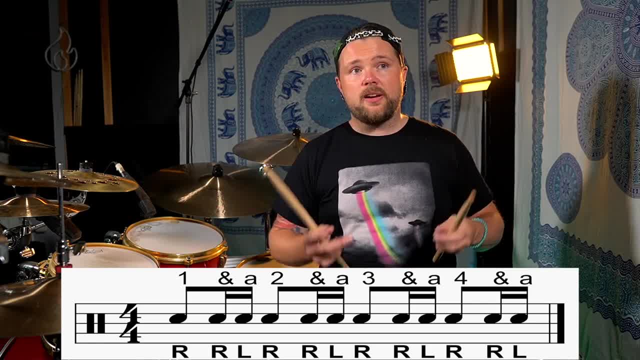 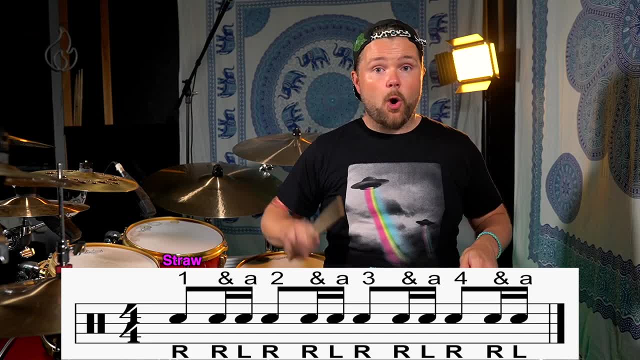 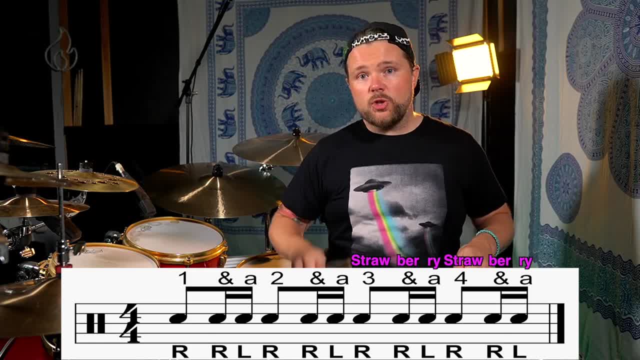 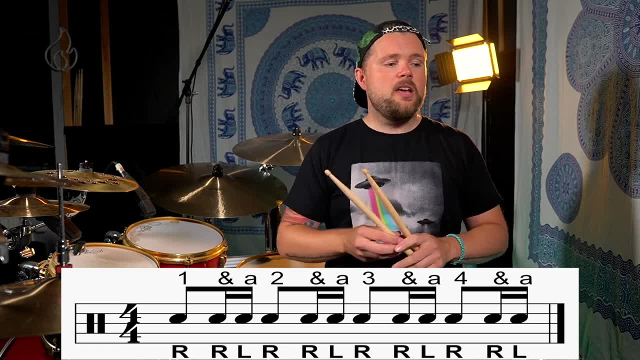 straw berry. It's the same thing: One and a, two and a straw berry, straw berry. See, You'll also notice that the sticking here is right, right, left, And that's because you should always have an underlying subdivision of sixteenth notes. So, since this rhythm starts with an eighth note, 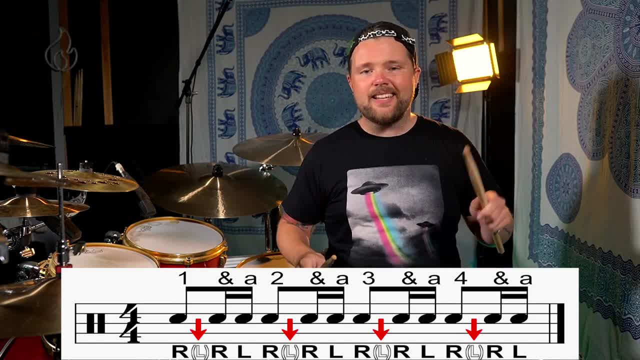 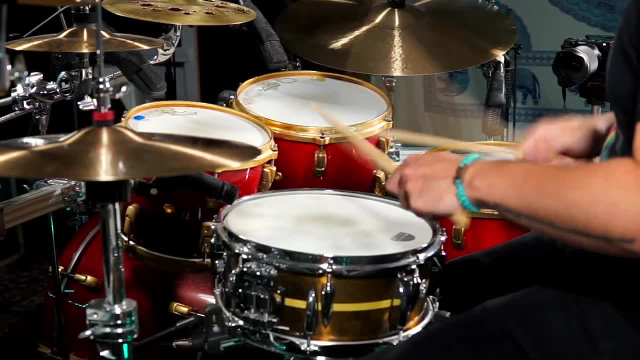 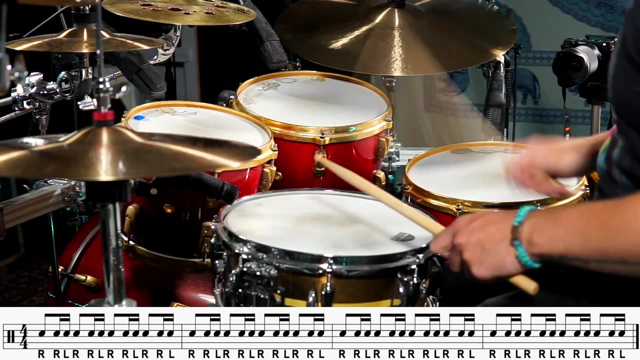 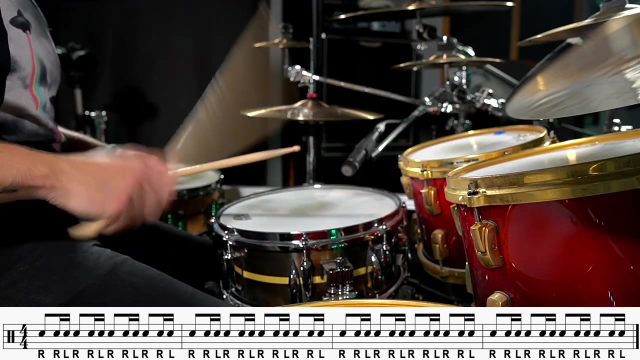 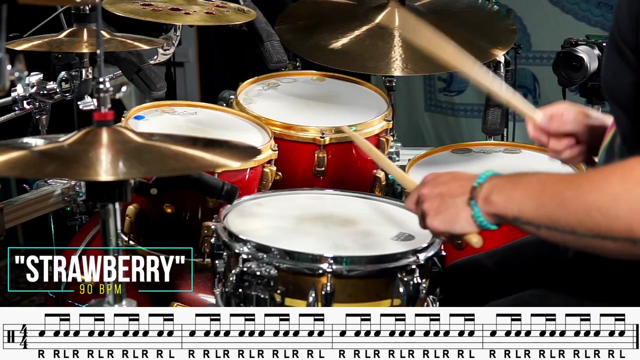 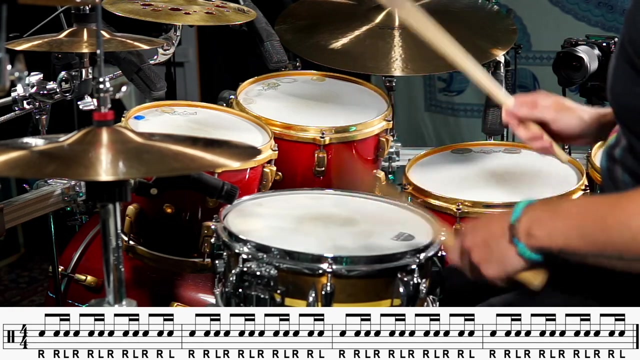 which is worth two sixteenth notes. you should imagine a silent sixteenth note in between, where the first left stroke would have been: Let's just try it out. So we'll say bing bing, bing, bing. Now we can start 54th note. 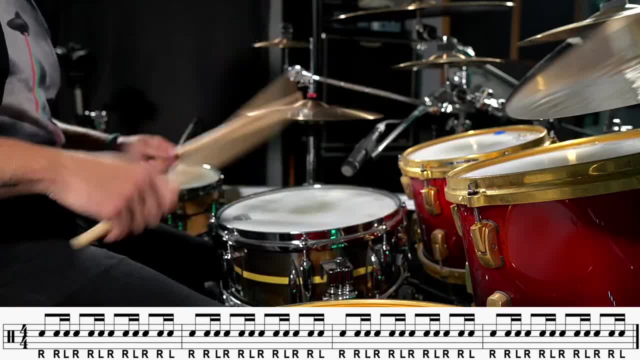 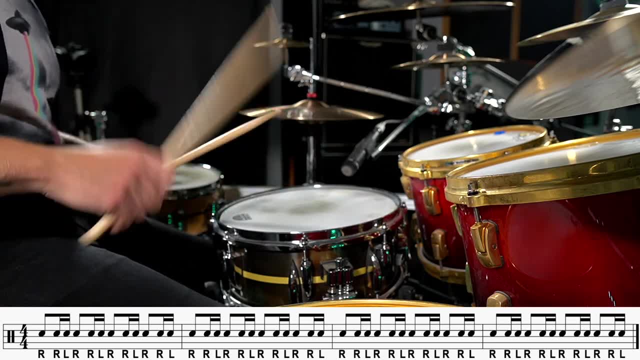 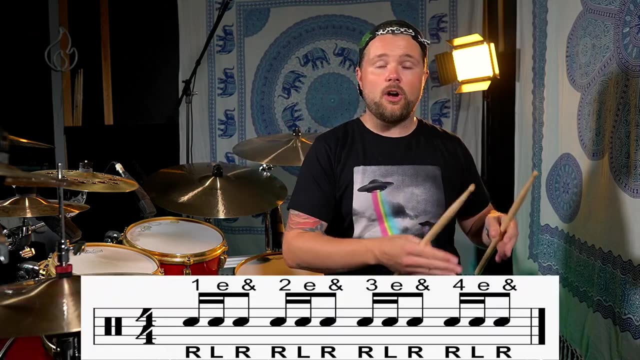 Okay, Now we can start 55th note and we'll go a little bit faster. We'll go about ten octaves and then we'll go from five octaves to six octaves, to a nine octaves, switch it around and start with the two sixteenth notes and end on the eighth note, When you count.